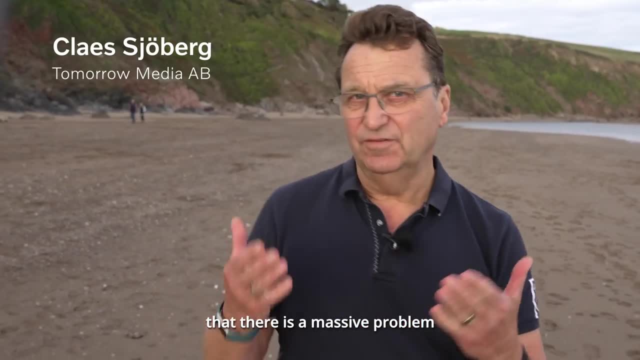 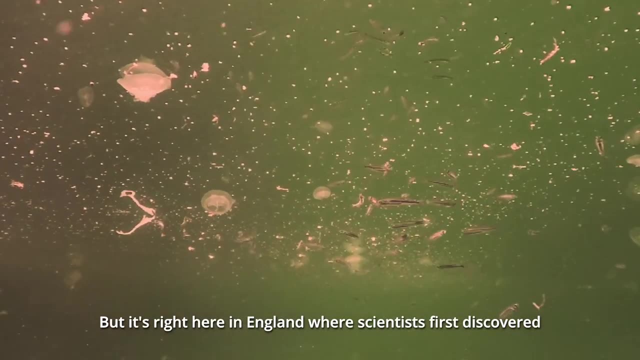 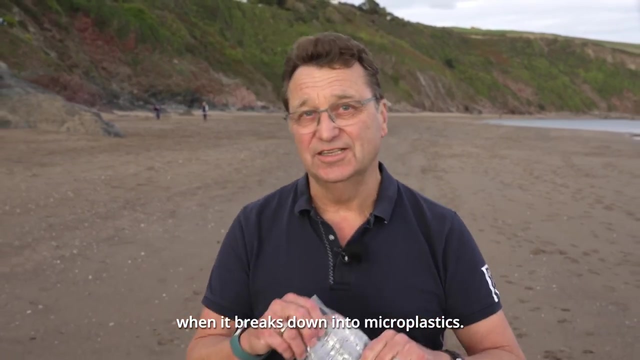 Looking at the sea from here, it's hard to understand that there is a massive problem of ocean plastic pollution out there. But it's right here in England, where scientists first discovered what happens to all our plastic waste when it breaks down into matter Microplastics. 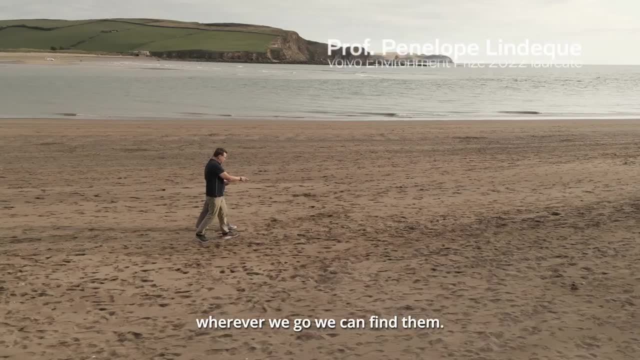 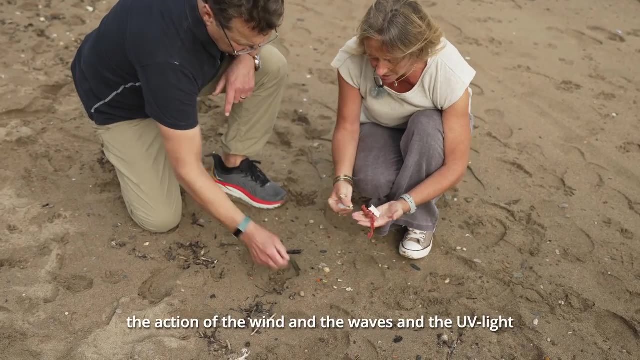 So microplastics are a huge array of contaminants. wherever we go, we can find them. Now, this is quite large plastic, as you can see, but when it's in the marine environment, the action of the wind and the waves and the UV light breaks it down into smaller and smaller. 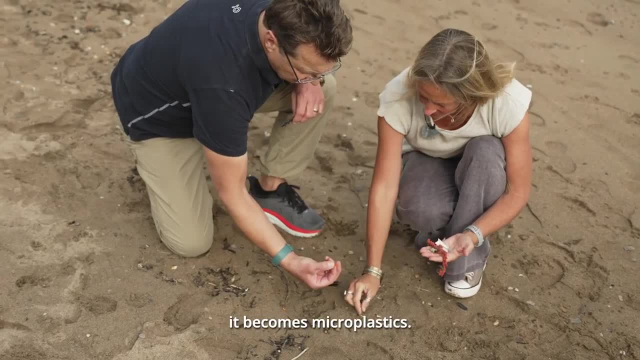 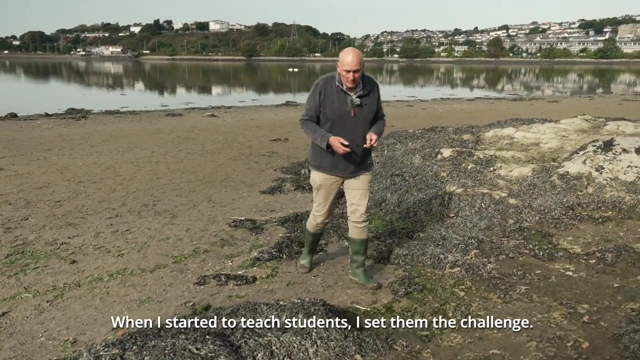 pieces. It doesn't degrade, it doesn't go away. it becomes microplastics. These small fragments are actually the most numerous. When I started to teach students, I set them the challenge. I said: go and find me the smallest piece of plastic on the beach. 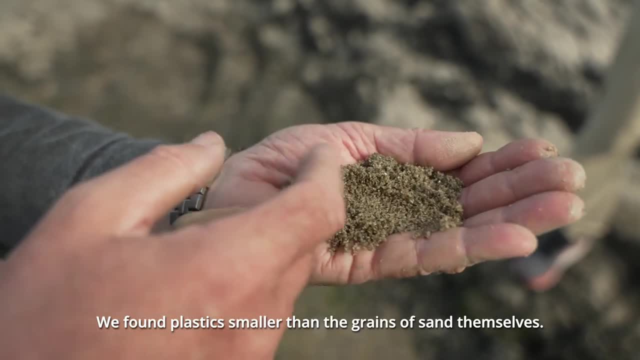 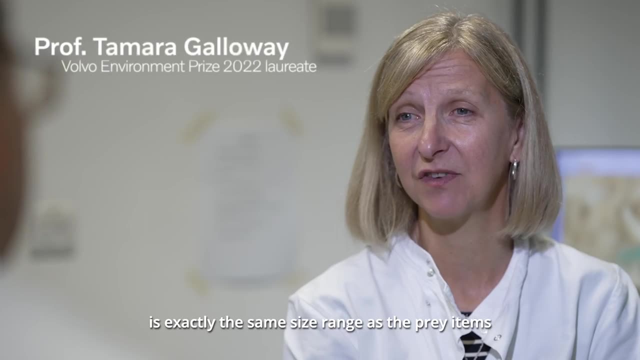 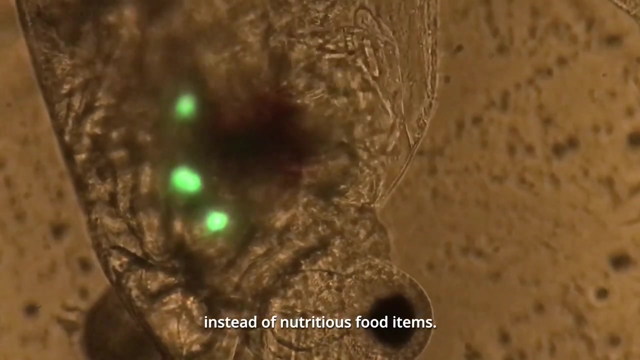 And that's really what started the story of the microplastics. We found plastic smaller than the grains of sand themselves. The size range that they break down into is exactly the same size range as the prey items for so many different marine animals, So there's the potential for them to be ingested instead of nutritious food items. 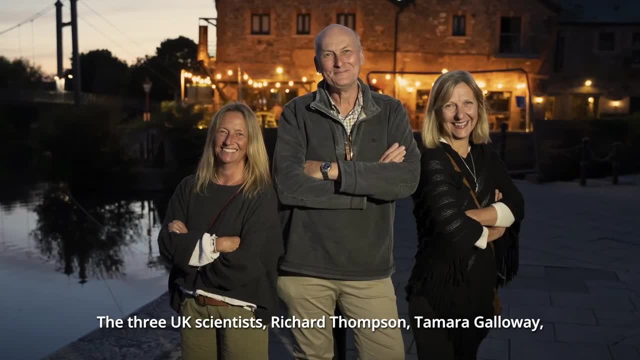 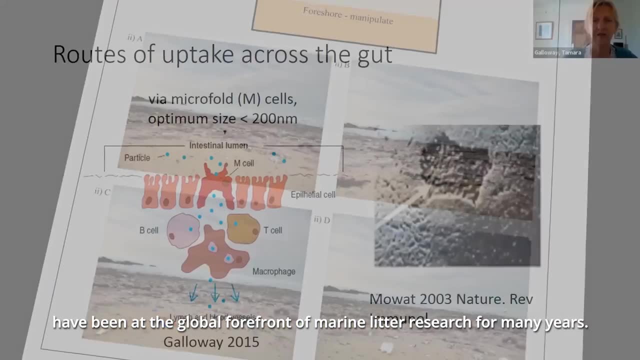 The three UK scientists Richard Thomson, Tamara Galloway and Penelope Lindigan have discovered the potential of microplastics. They have been at the global forefront of marine litter research for many years. They have also helped to bring about changes in global policy with their work central. 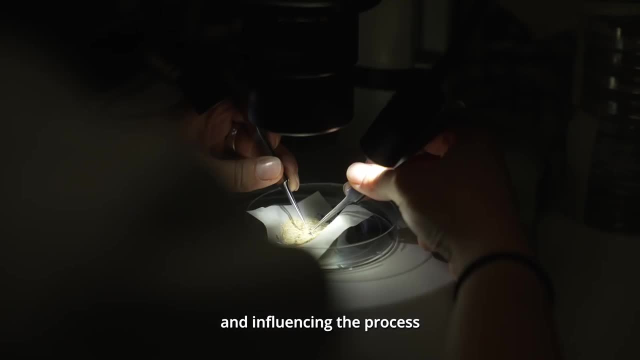 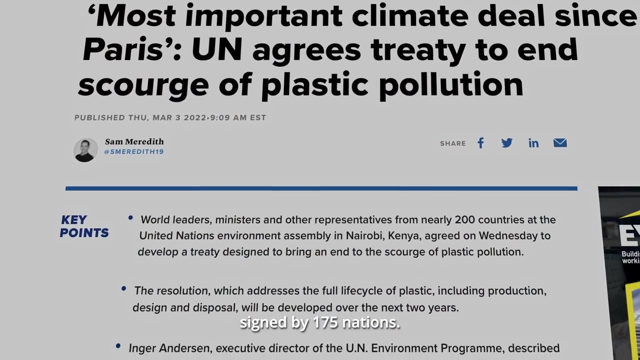 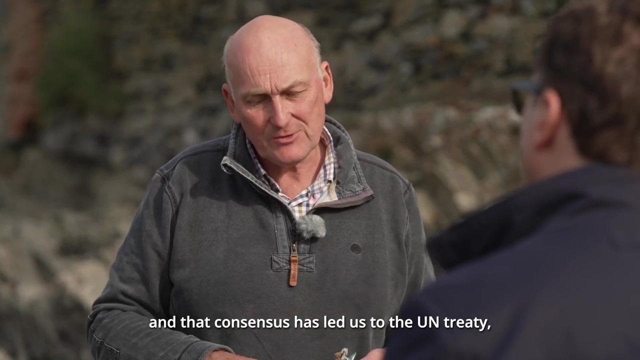 to international government legislation and influencing the process leading to the United Nations Treaty on Plastic Pollution, signed by 175 nations. I think everybody is actually on the same page, that there is a problem and that consensus, I would say, has led us to the UN Charter. 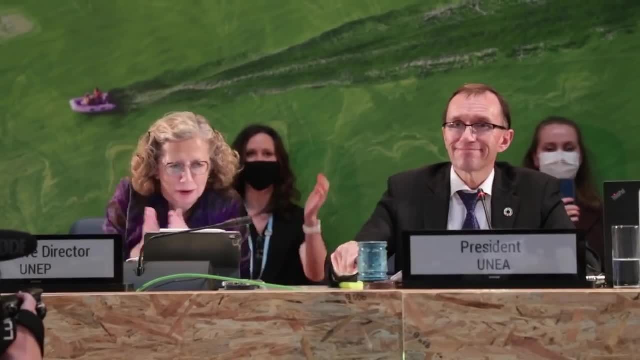 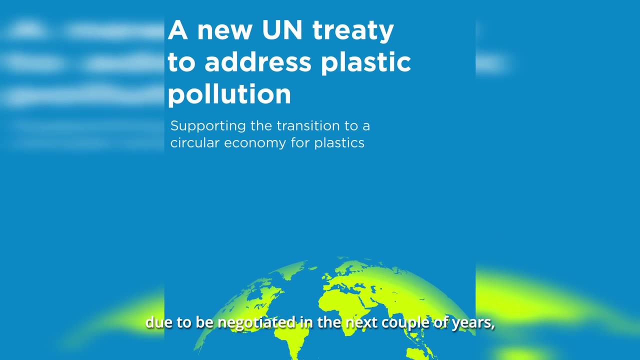 I think everybody is actually on the same page, that there is a problem, and that consensus, I would say, has led us to the UN Charter, Which is fantastic, The UN treaty on plastic pollution due to be negotiated in the next couple of years. 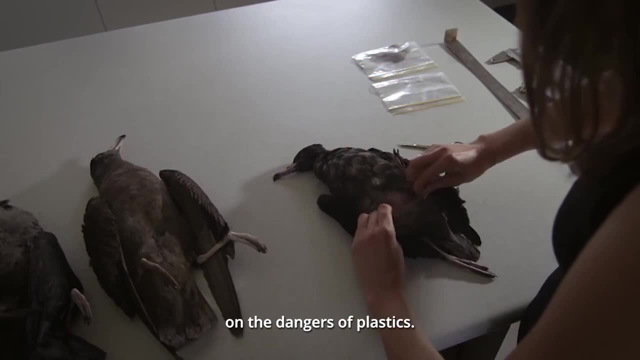 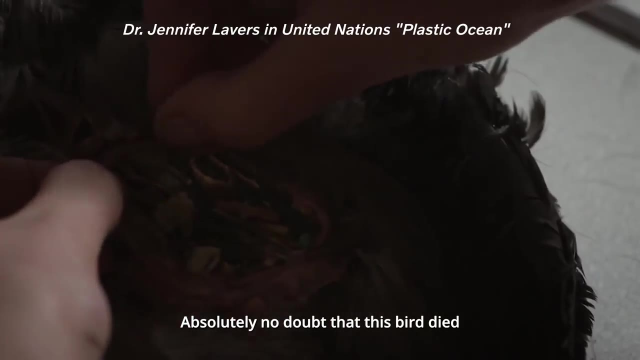 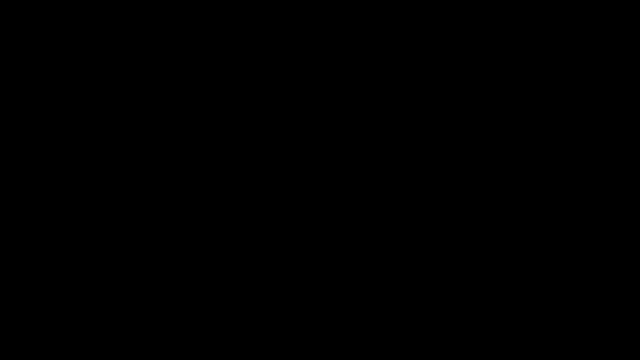 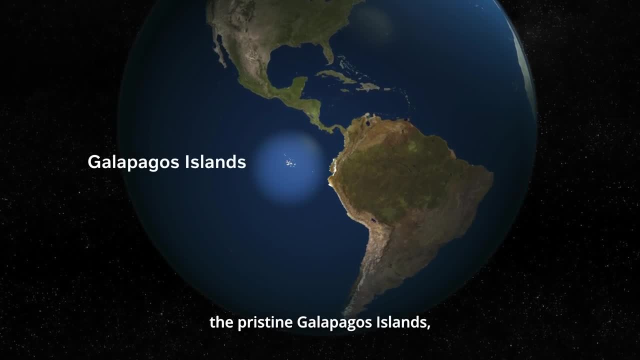 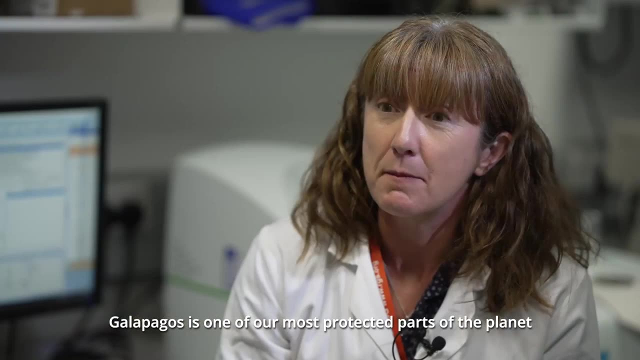 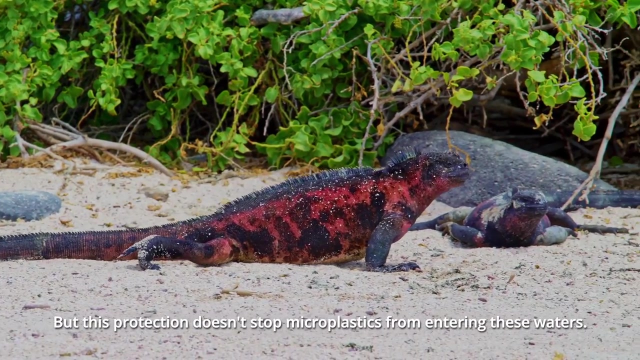 It's awful. world's most protected natural environments, the pristine Galapagos Islands, scientists find vast amounts of microplastics. Galapagos is one of our most protected parts of the planet for the marine environment. That protection is what gives us this great biodiversity. But this protection doesn't. 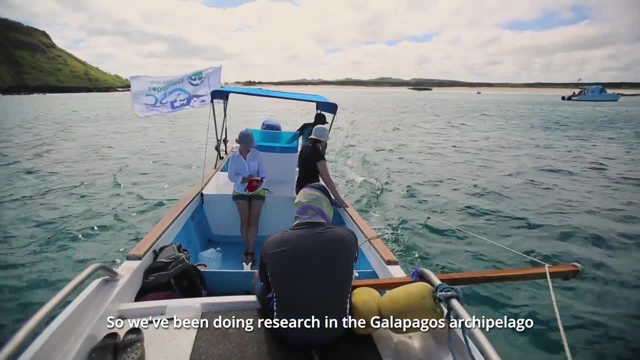 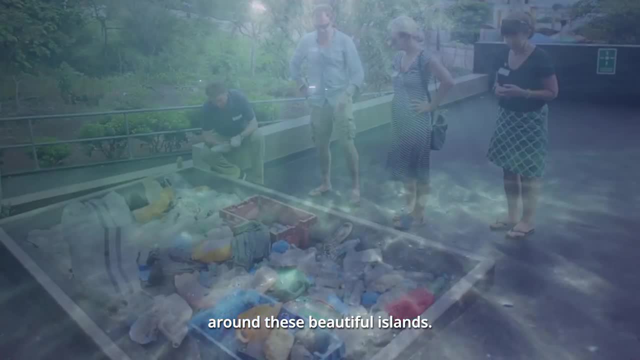 stop microplastics from entering these waters. So we've been doing research in the Galapagos archipelago for the last three years and we've found quite high numbers of microplastics around those beautiful islands. These are our samples from the Galapagos, So we bring it back here to the lab where 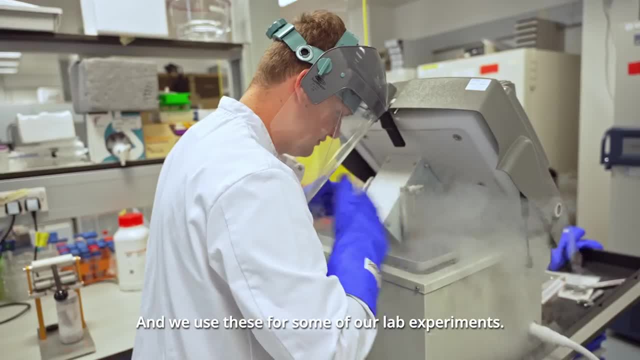 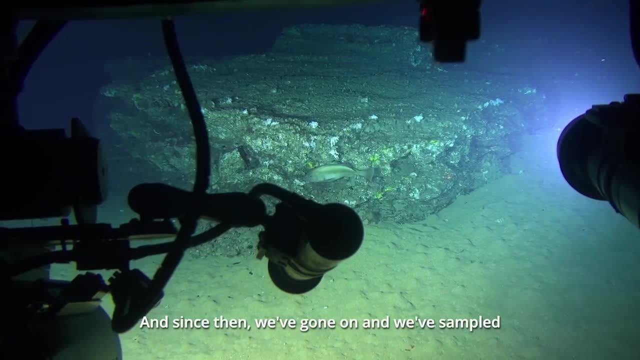 we sort the plastics as you can see here, And we use these for some of our lab experiments. We've collected samples from the deep sea, working with deep sea biologists, And since then we've gone on and we've sampled samples of snow taken from Everest and we're finding 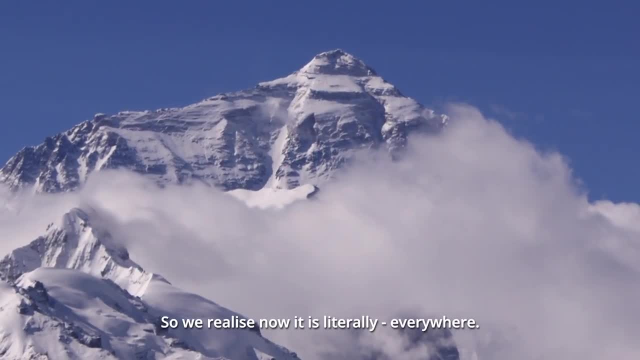 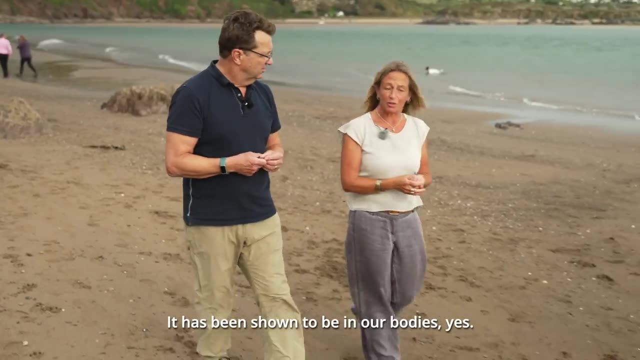 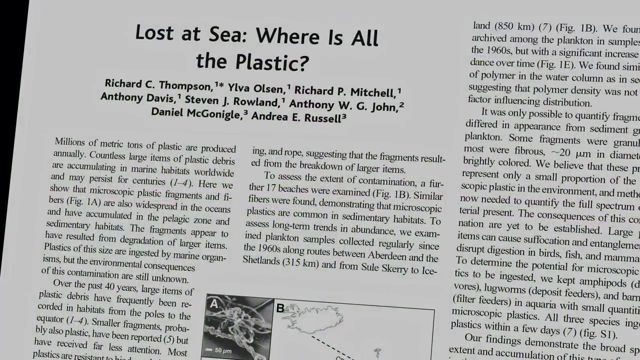 microplastic there that's ridged it by the air, So we realise now it is literally everywhere. Do humans have it in our bodies too? It has been shown to be In our bodies, yes, Even to the fact that it's been in the placenta of pregnant women. 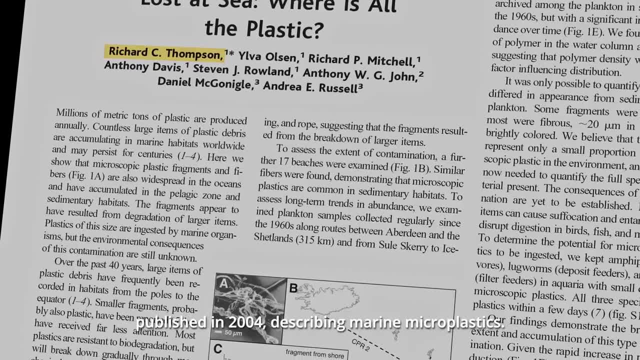 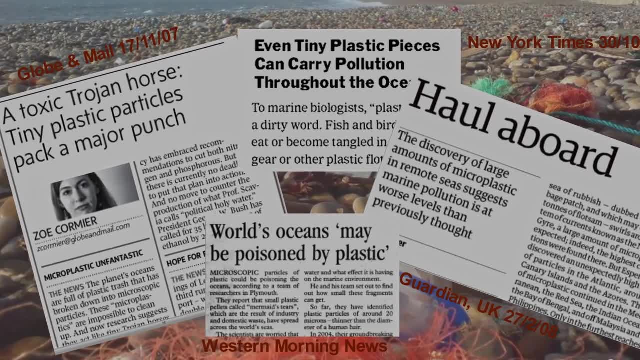 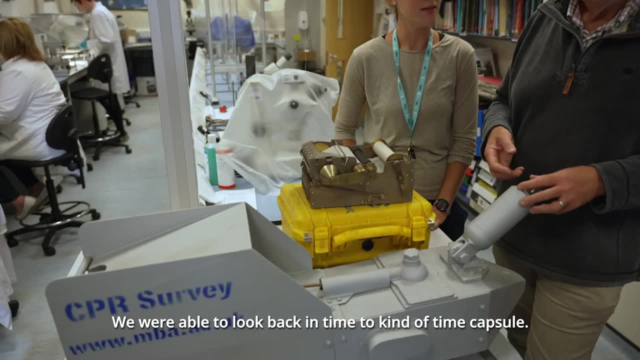 Richard Thomson led the first study, published in 2004,, describing marine microplastics. It was an alarm bell that got a lot of attention and the topic has since become a focus for research worldwide. We were able to look back in time at a kind of time capsule and we showed actually comparing- 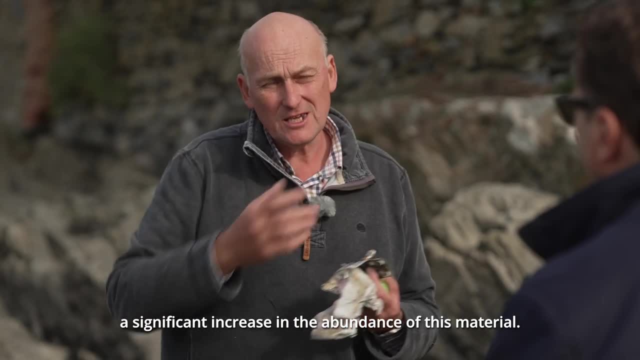 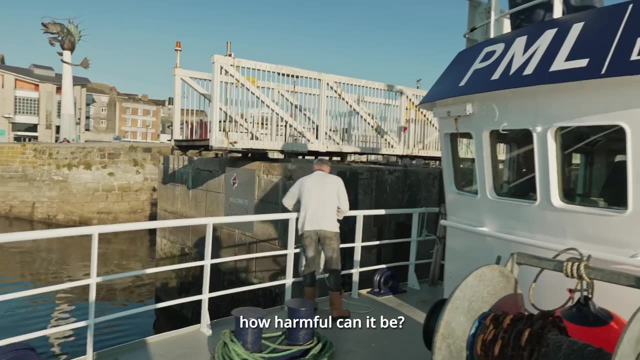 across the decades, over 40 years- And we found that actually a lot of microplastics are in the ground, And we've seen the increase in the abundance of this material. So then, the next steps were almost to go on and look at the, the. so what question, if you like, how harmful can it be? 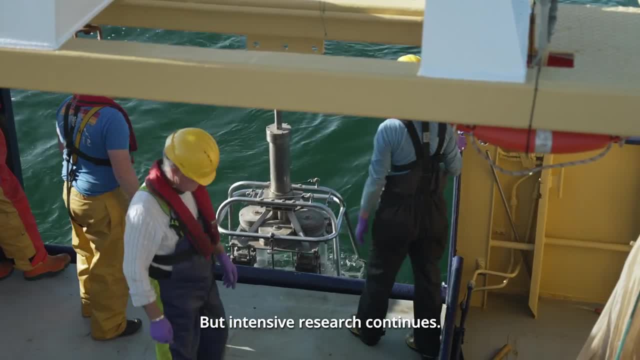 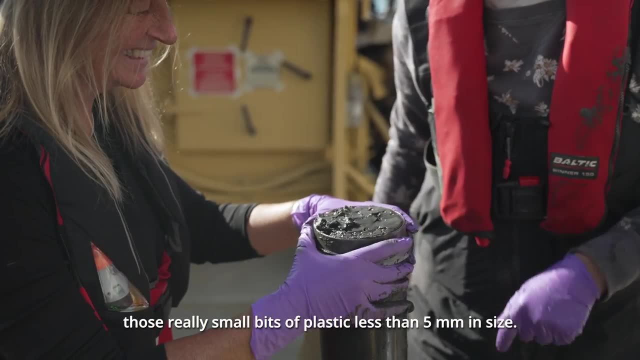 There are still significant gaps in knowledge about how microplastics spread and where they go, But intensive research continues. What we're doing is we're sampling from microplastics Those really small bits of plastic less than five millimetres in size. 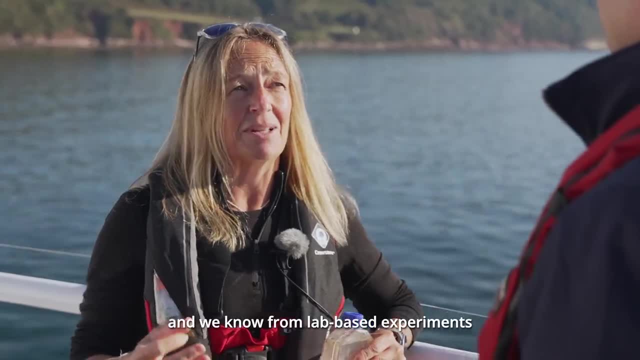 We want to know how much is in the marine environment. We're also sampling for zooplankton And we know that microplastics are very important for the environment. The X-rays are really important. know from lab-based experiments that nearly every zooplankton species we've 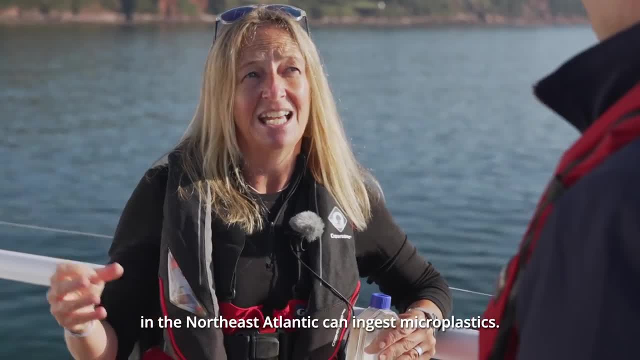 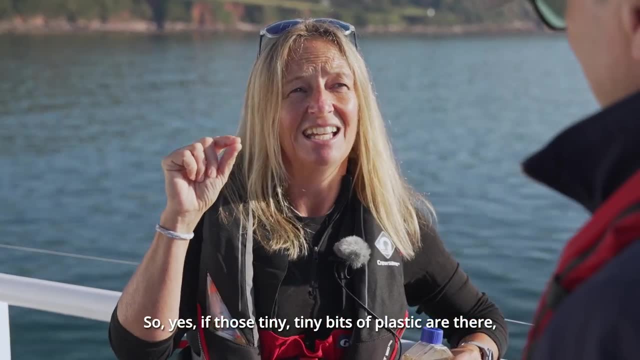 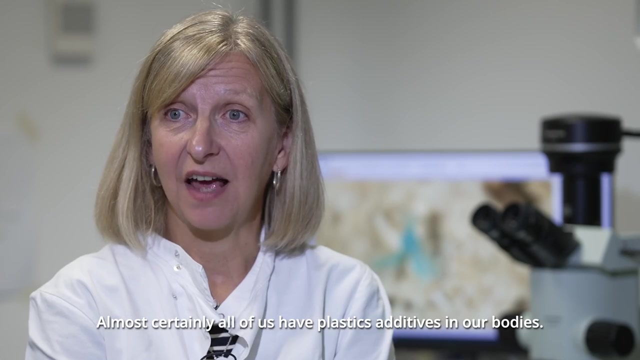 looked at in the Northeast Atlantic, can ingest microplastics, and we now know that that also happens in the natural environment. so yes, if those tiny, tiny bits of plastic are there, then the zooplankton can eat them. almost certainly all of us have plastics additives in our bodies. we know that. for 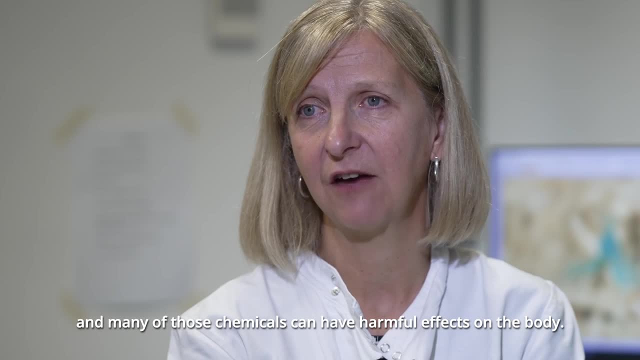 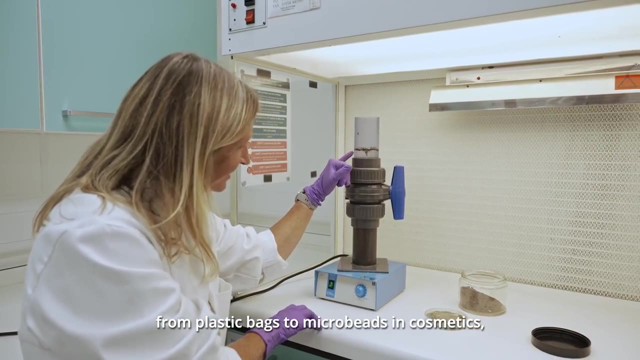 many of the studies that have been going on. for some, many of those chemicals can have harmful effects on the body. the scientists have also tracked the sources, from plastic bags to microbeads in cosmetics and tire particles. it's clear that tires wear on the road and they generate particles. what wasn't clear was 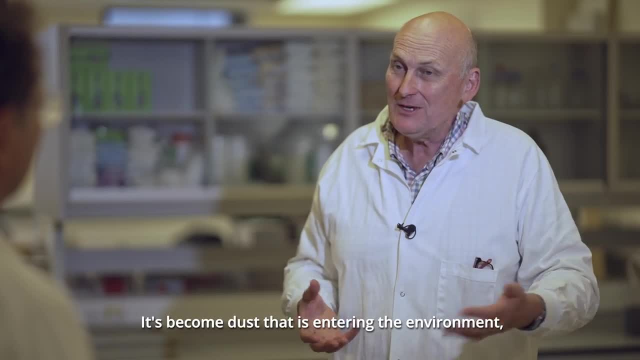 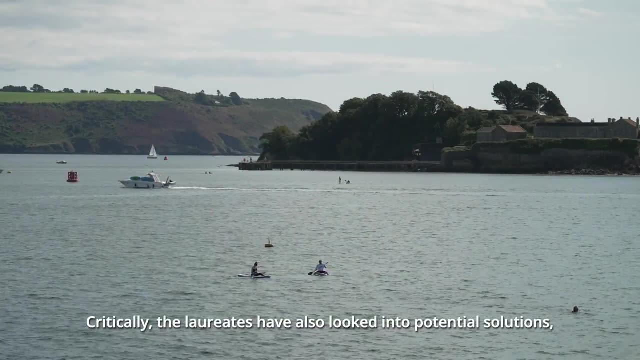 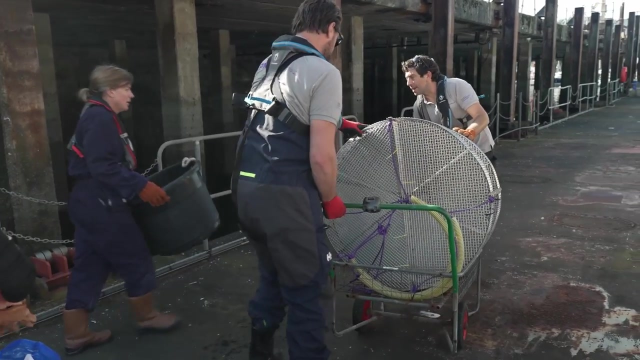 where do they go? it's become dust that is entering the environment, entering watercourses, entering the oceans critically. the laureates have also looked into potential solutions, evaluating the potential for natural and mechanical measures to clear plastic from the ocean environment. one of the things we're doing is turning towards a nature-based 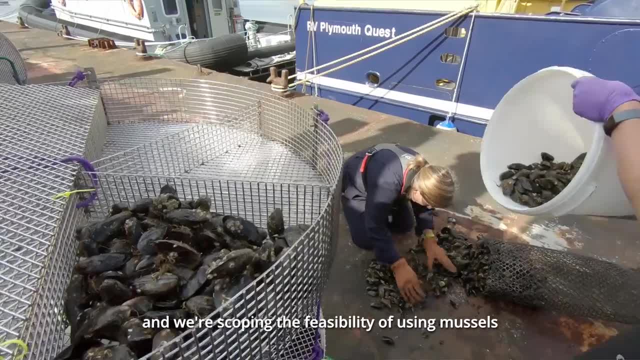 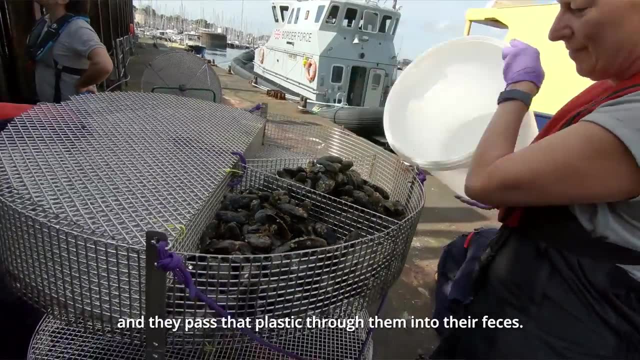 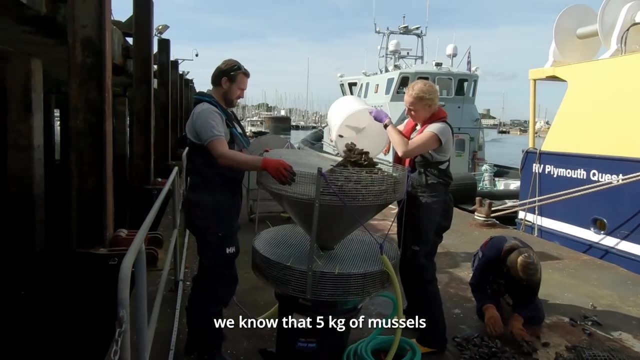 solution and we're scoping the feasibility of using muscles, which are natural filter feeders and they can ingest the plastic as they ingest their normal food and they pass that plastic through them into their feces. and from our lab-based experiments we know that five kilograms of muscles can remove a 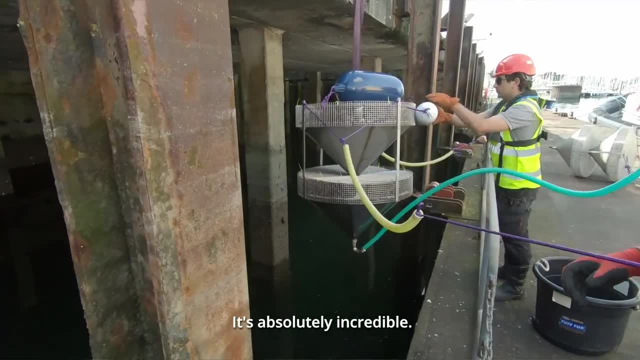 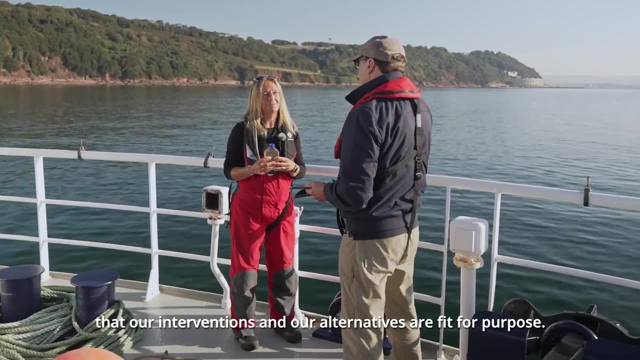 quarter of a million plastics per hour. it's absolutely incredible. so we do a lot of testing to make sure that the plastic that we ingest is actually sustainable and that we can make sure that our interventions and our alternatives are fit for purpose. but then there are other sources of 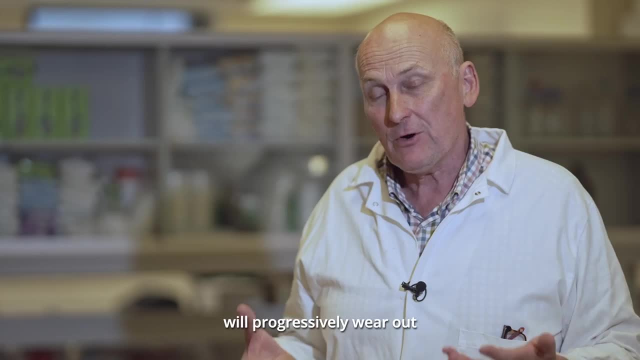 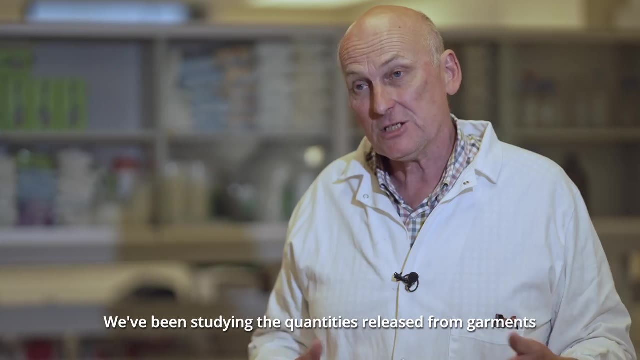 fragmentation, from where that all of the textiles, the clothing we're wearing, will progressively wear out whilst we're walking around in it, using it, but especially also while we're washing it. we've been studying the quantities released from garments as you wash them and how that varies according to the 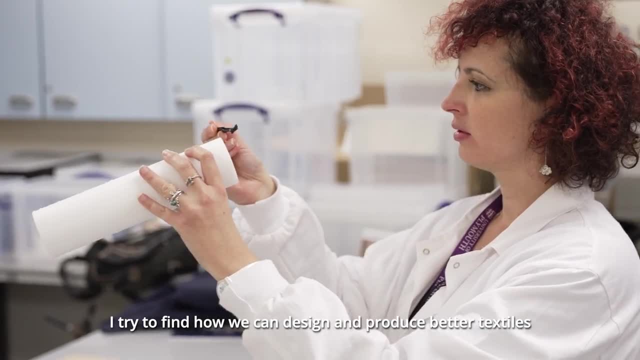 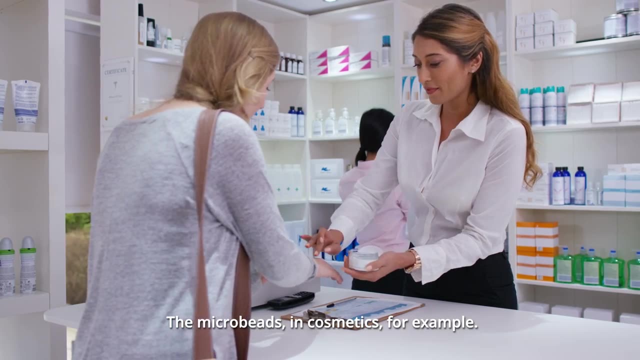 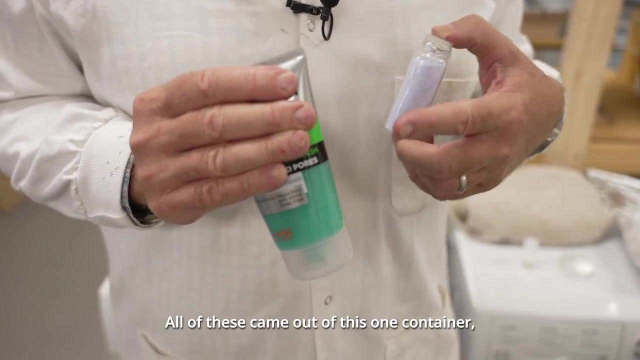 style of the garment. I try to find how we can design and produce better textiles to reduce the amount of microfibres that are released to the environment. the microbeads in cosmetics, for example- very small particles used in cosmetics as an abrasive agent. all of these came out of this one container. in fact, some of the 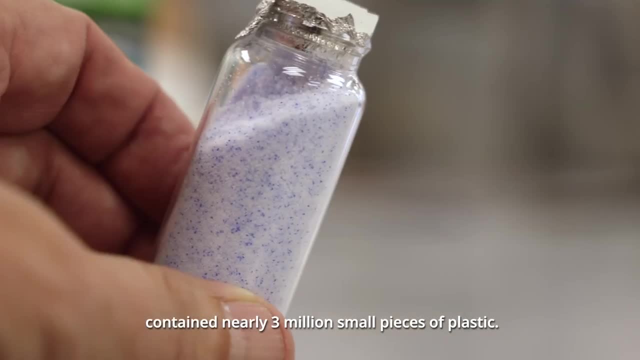 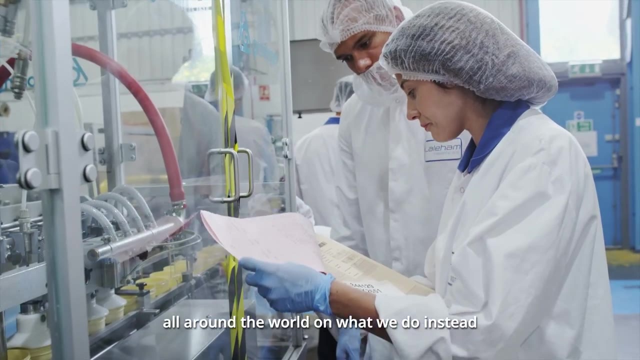 containers we looked at contain nearly three million small pieces of plastic. there's a huge effort going on in research and innovation all around the world on what we do instead and how we can produce safer alternatives. the problem is it's a design problem. we're designing plastics to be robust and 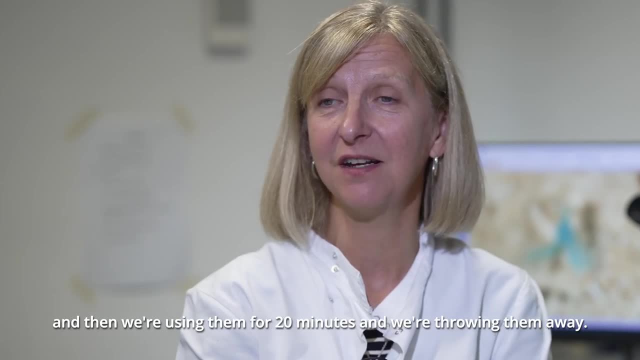 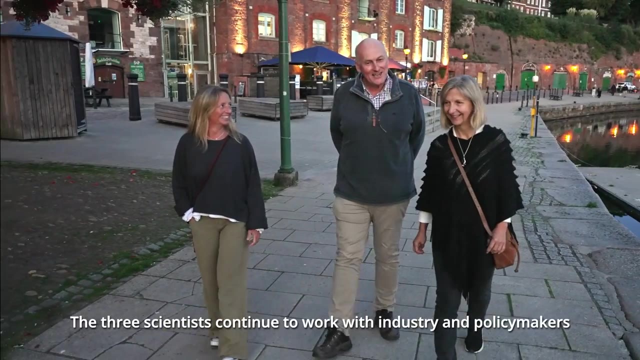 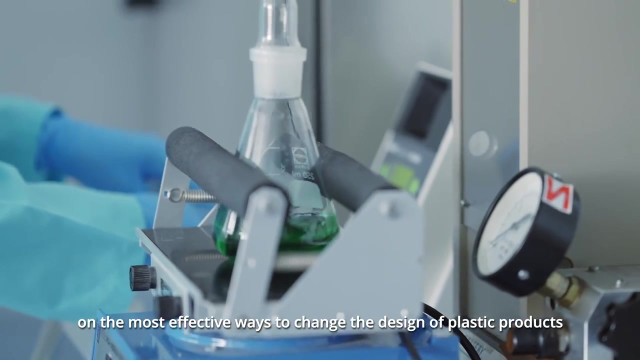 to survive for 500 years, and then we're using them for 20 minutes and we're throwing them away. I mean it's not a surprise that we've got a problem. the three scientists continue to work with industry and policymakers on the most effective ways to change the design of plastic products and to bring about a 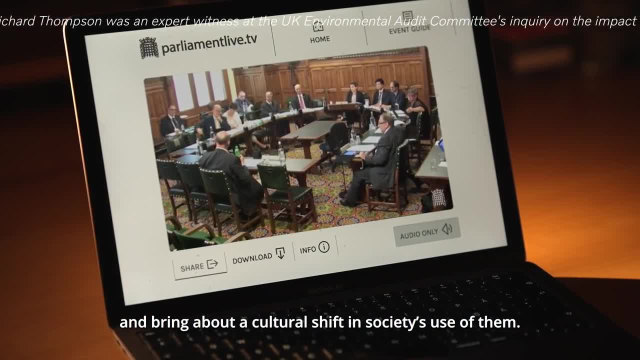 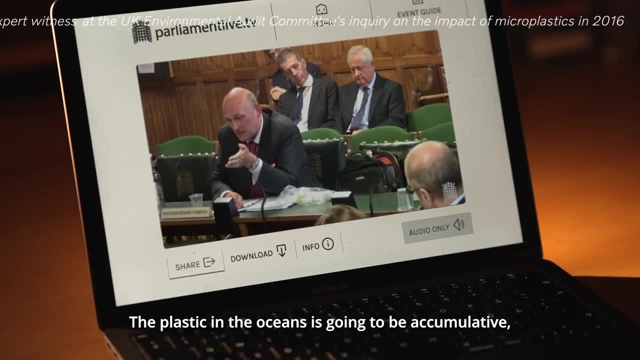 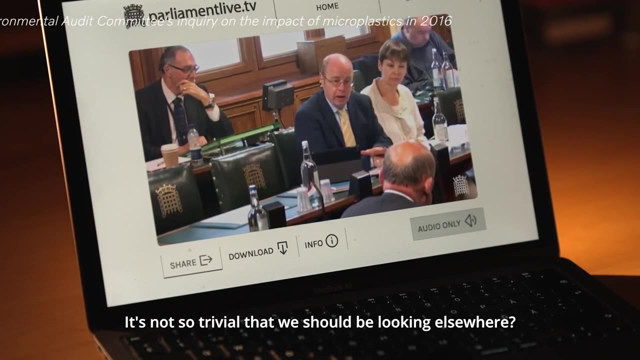 cultural shift in society's use of them. you are perhaps the the godfather of micro plastics, and how far is our knowledge developed? the plastic in the oceans is going to be cumulative. it's not going to biodegrade. it is worth tackling. it's not so trivial that we should be looking elsewhere, you know, but certainly we. 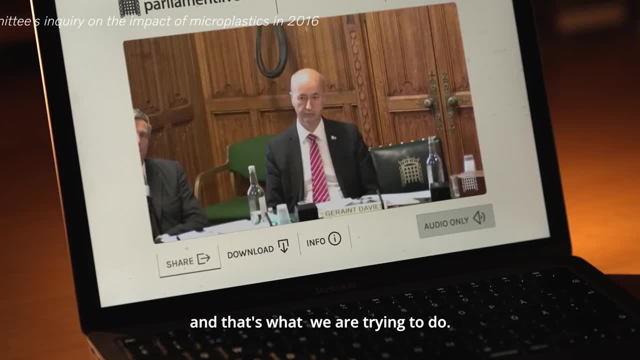 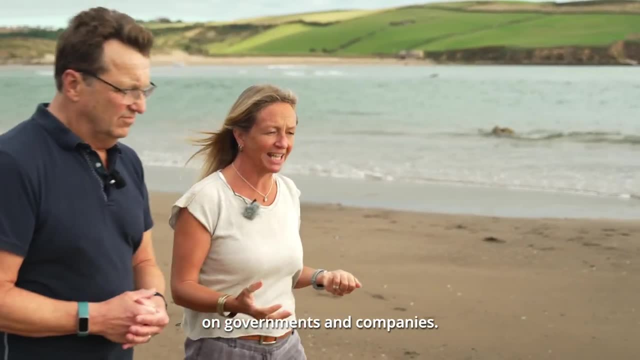 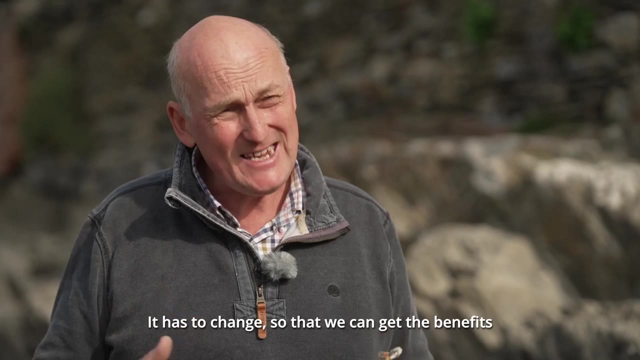 realize there's a need to gather more evidence on harm, and that's what we're trying to do. we've educated the public and that's helped put pressure on governments and companies. what about the process that gives them no alternative to use a plastic that will degrade harmlessly? it has to change so that we 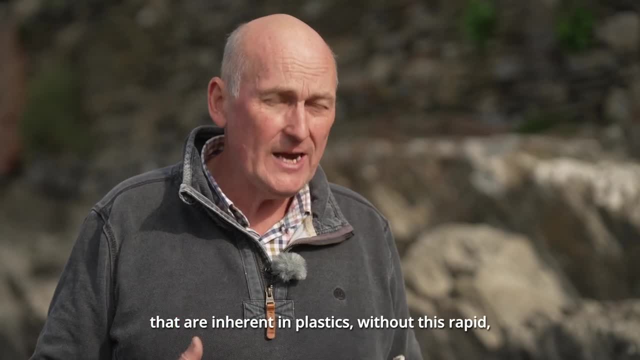 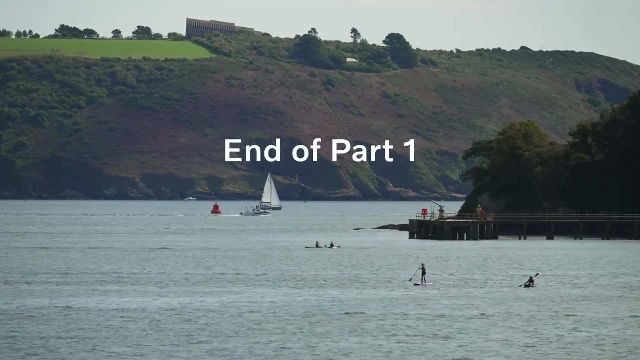 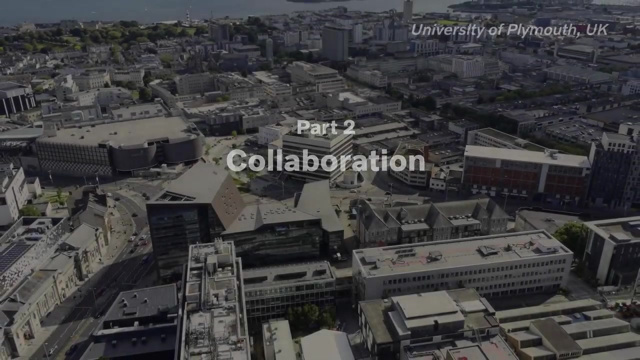 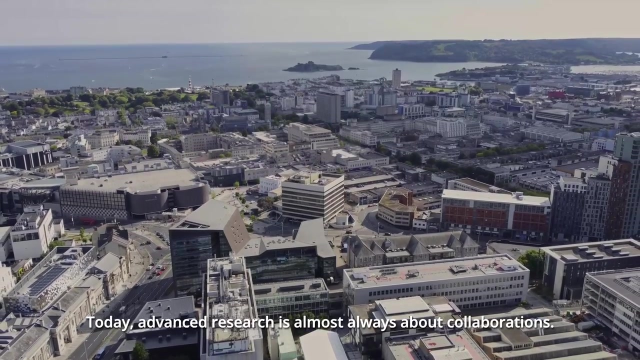 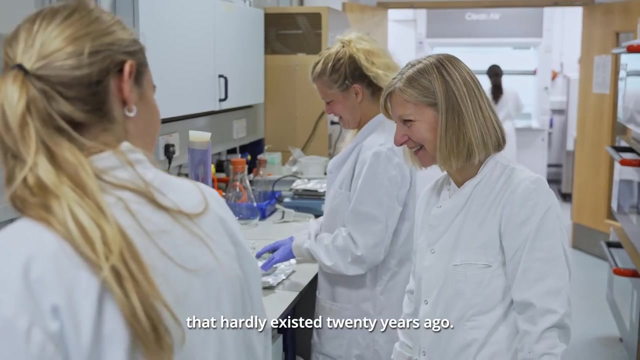 can get the benefits that are inherent in plastics without this rapid, continuous accumulation of highly persistent waste. today, advanced research is almost always about collaborations. the three award winners have succeeded in developing methods and results within a research area that hardly existed 20 years ago. in many ways, you could say we're quite similar: we've got passion, we've got drive. 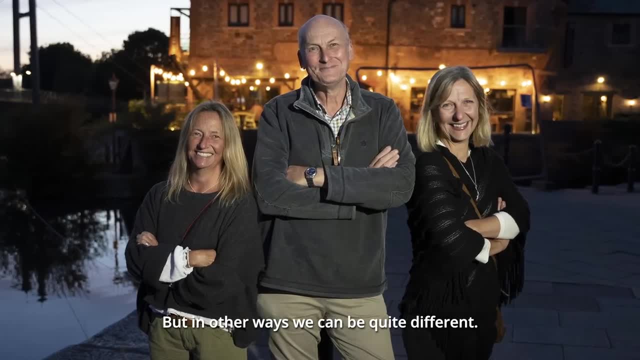 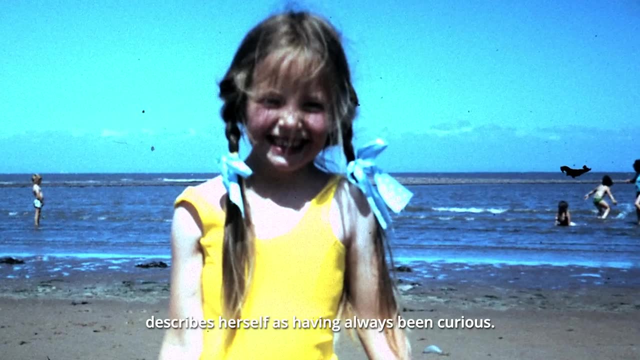 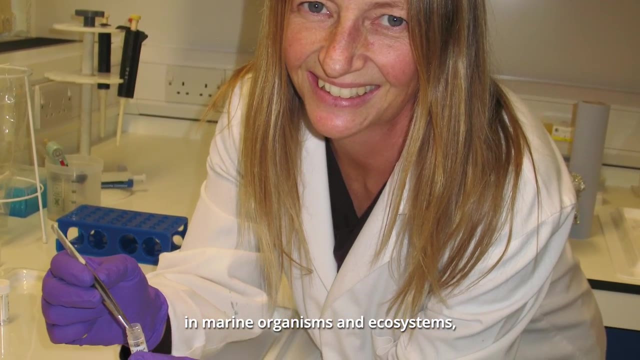 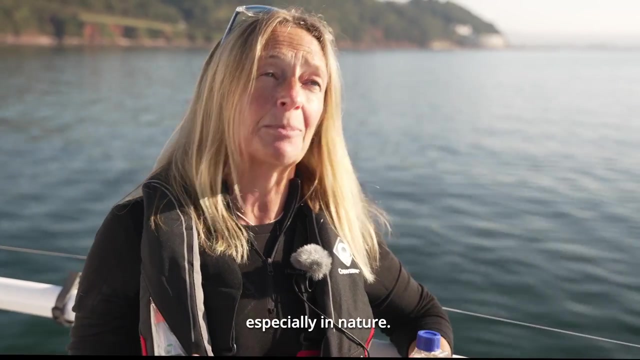 we've got curiosity, but in other ways we can be quite different. Penelope Lindegue, born and raised in South Devon, describes herself as having always been curious. her fascination with biology led her to a scientific career in Marine organisms and ecosystems, particularly zooplankton. I've always been intrigued about understanding how things work. 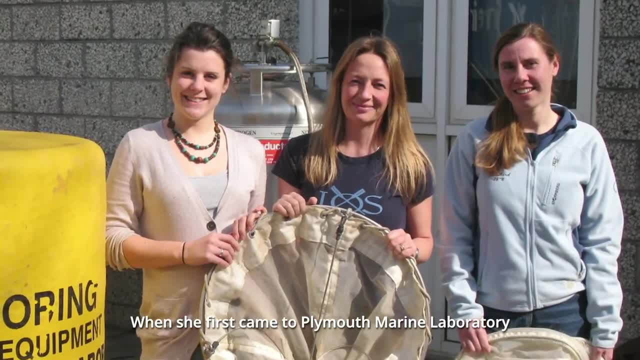 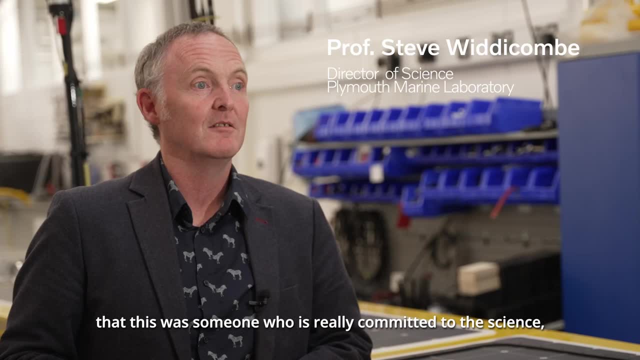 When she first came to Plymouth Marine Laboratory she was a PhD student looking at zooplankton and I knew right from the very start that this was someone who was really committed to the science but also to the environmental cause that underpins that science as well. I became interested in 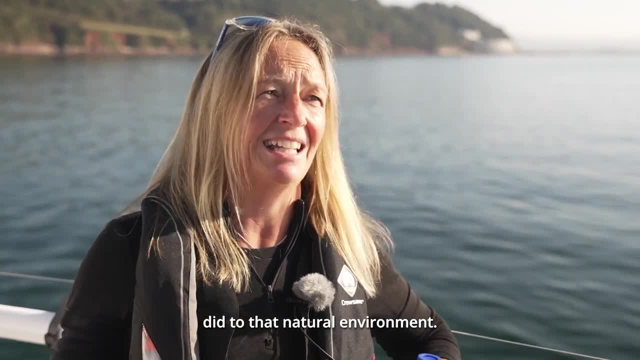 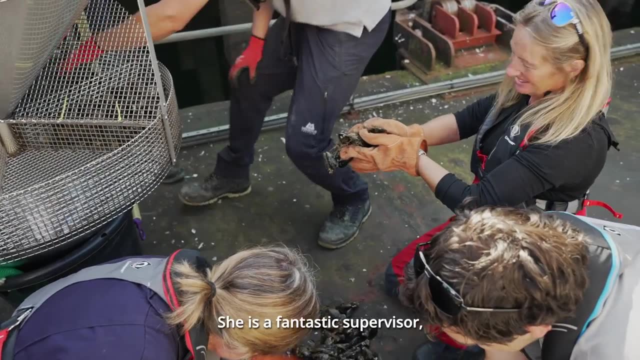 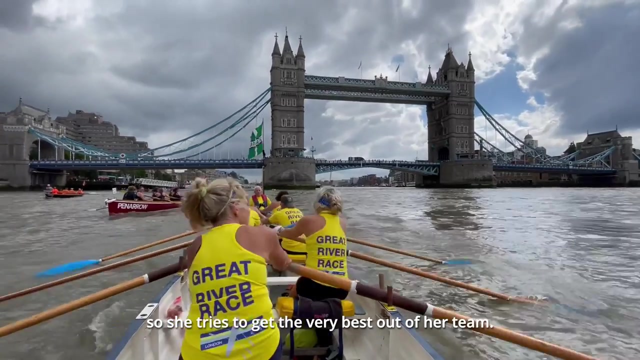 knowing what we, as humans, did to that natural environment. what impact did we have, in particular, on anthropogenic pollutants? She is a fantastic supervisor, making sure that we have a good work-life balance, so she tries to get the very best out of her team. 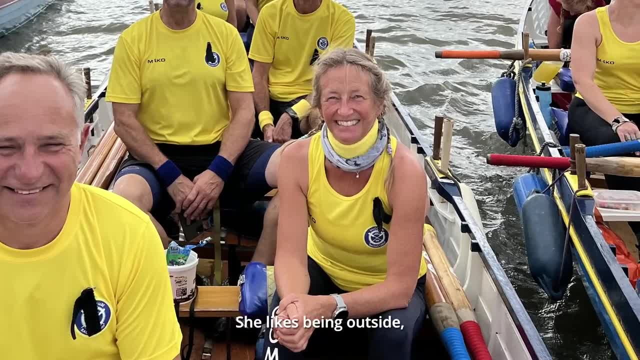 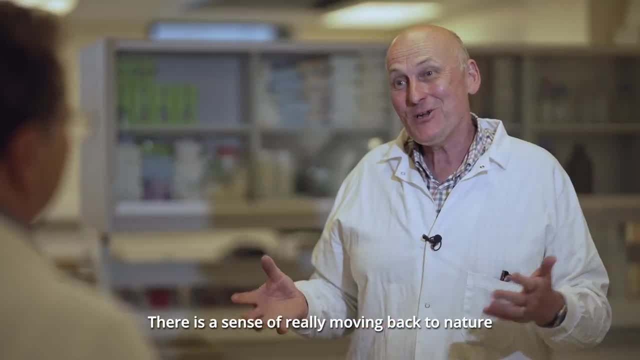 Penny is very good at all sports. She likes being outside. she just loves being on a paddleboard. she loves being outside in the ocean. There's a sense of really moving back to nature and farming and being self-sufficient. that's really really close to her heart. 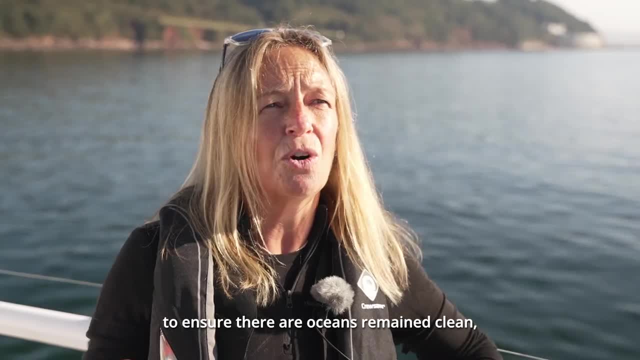 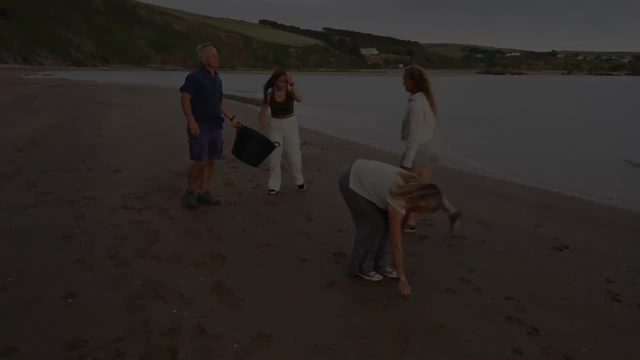 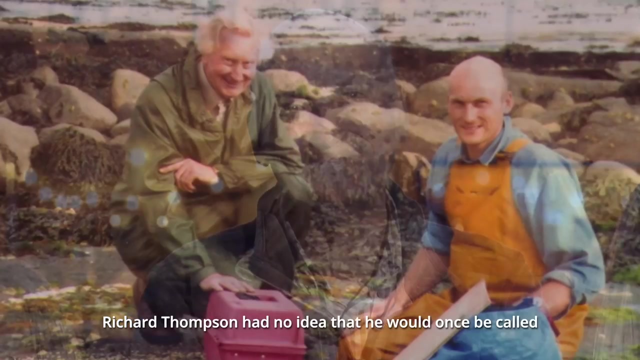 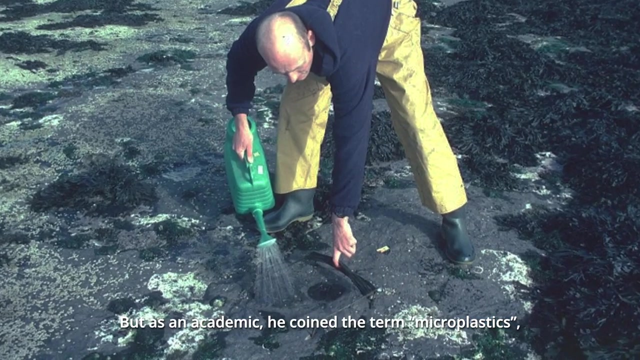 I want to make a difference to ensure that our oceans remain clean and productive and healthy for our children and our children's children. When studying to become a marine biologist, Richard Thompson had no idea that he would once be called the godfather of microplastics, But as an academic he coined the term microplastics. 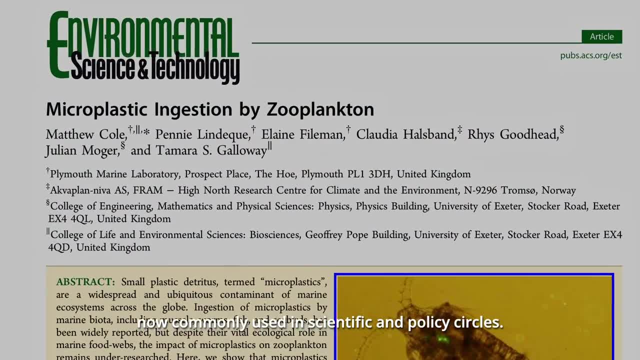 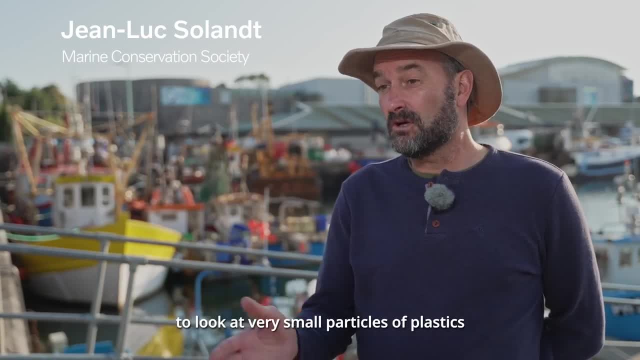 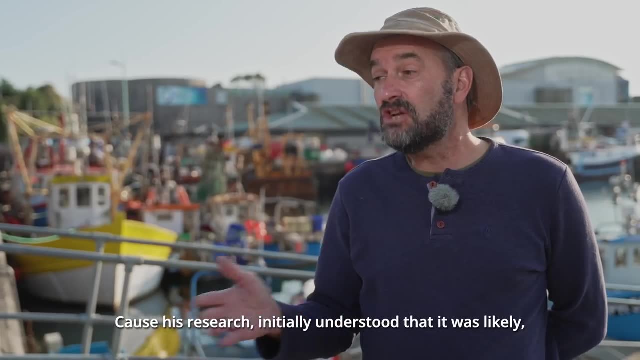 now commonly used in scientific and policy circles. Richard was fundamentally fundamental to adjusting our survey methodology in about 1990 to look at very small particles of plastics which were going to very soon degrade into microplastics, because his research initially understood that it was likely at that point in time to go into the food chain. So he was. 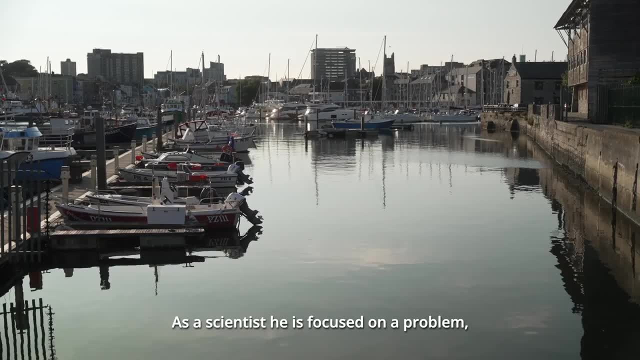 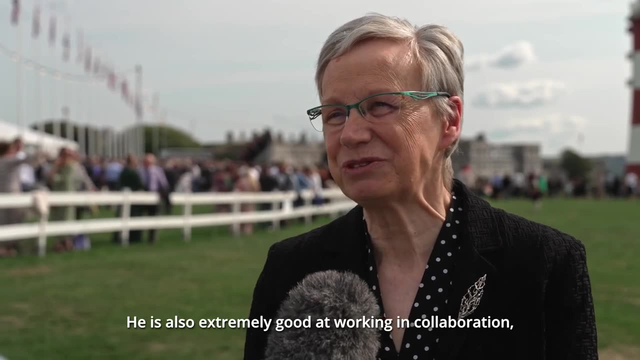 fundamental to how we worked. As a scientist, he's focused on a problem and until he's solved the problem, he won't give up. He's also extremely good at working in collectives. He's particularly interested in collaboration and he's particularly interested in how do you deal? 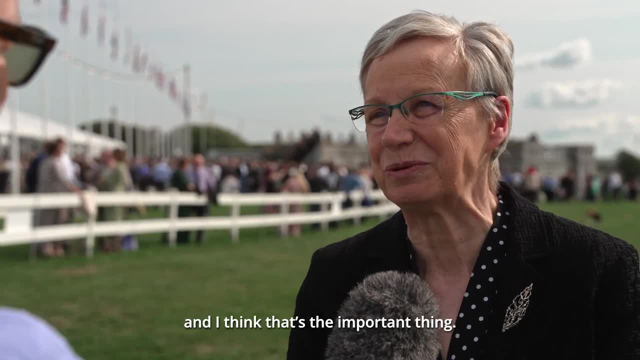 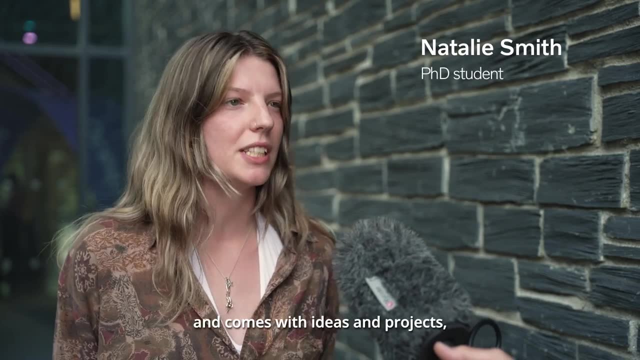 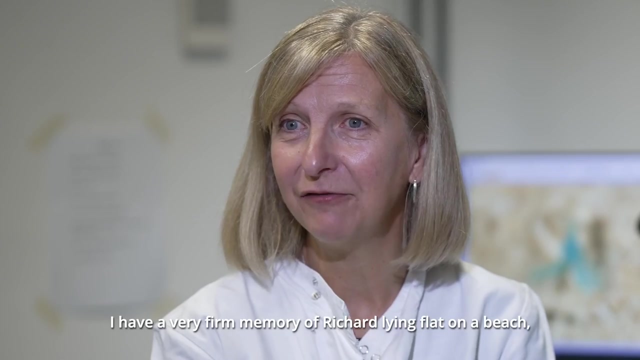 with the outcome, not just what is the outcome, and I think that's the important thing. People's minds work differently and the way he thinks and the way he processes stuff and comes up with ideas and projects is just really inspiring and really amazing. When we went to the Galapagos island, I have a very firm memory of Richard lying flat. 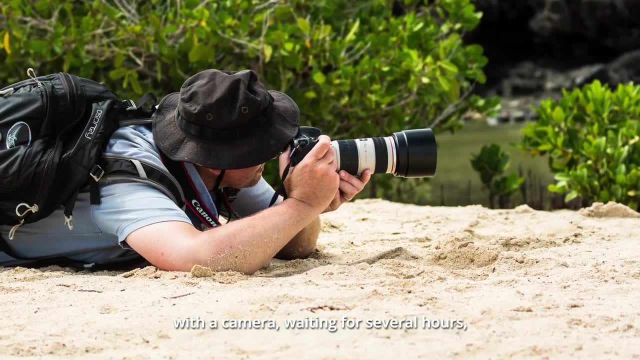 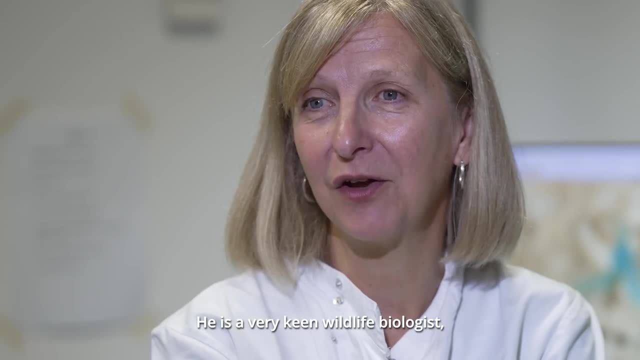 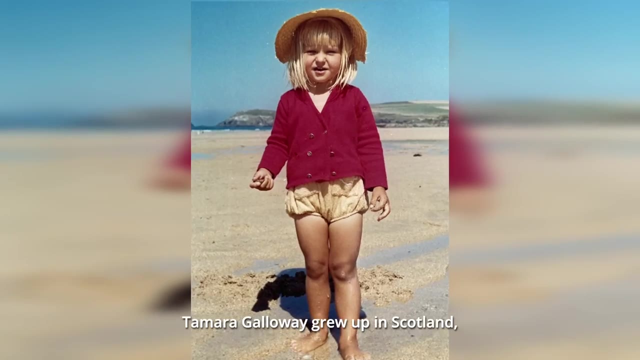 on a beach with a camera, waiting for several hours for a Galapagos flamingo to do something. He's a very keen wildlife biologist and very patient. I couldn't have done that. Tamara Galloway grew up in Scotland and studied biochemistry at the universities in Glasgow and